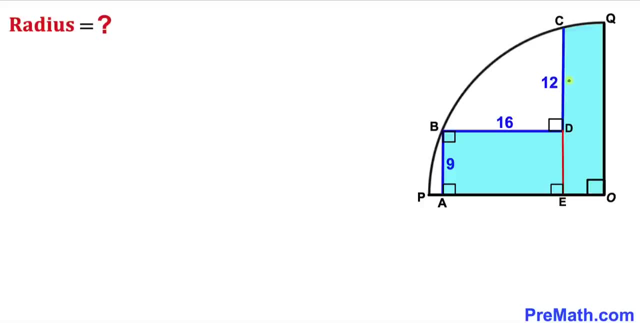 And here's our very first step. I have extended this segment CD all the way to this point E and, as a result, we got this rectangle ABDE, and in this rectangle this side length AB is going to be equal to this side length DE, and likewise, this side length BD is going to be equal to this side length AE. 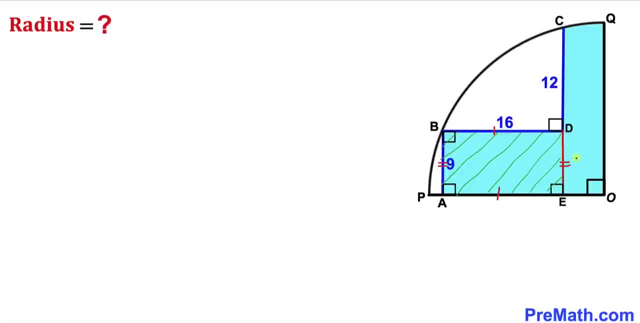 So, therefore, this side length DE is going to be 9 units, whereas this side length AE is going to be 16. and in this next step I have connected this center O with this point B and now we can see that this OB is the radius of this quarter circle. Let me label this radius as our lower case R, and now we know that this segment E is going to be equal to this side length DE. 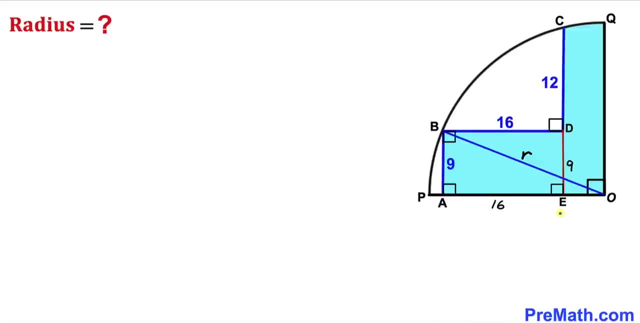 So therefore, this side length AE is 16, and now let's assume that this tiny segment EO is A, then this whole length AO is going to be 16 plus A. and here, in this next step, I have connected this center O with this point C and we can see that this OC is the radius of this quarter circle. 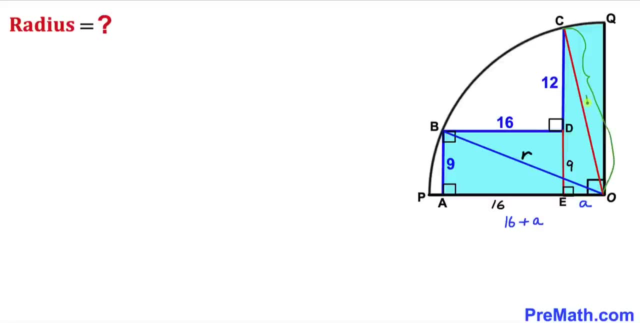 So, therefore, I'm going to label this radius as lower case R as well. and here's our next step. Let's focus on this right triangle, OAB, whose side lengths are 9 radius R and 16 plus A, and now we are going to apply the Pythagorean theorem. and here's our Pythagorean theorem: A squared plus B squared, equal to C squared. 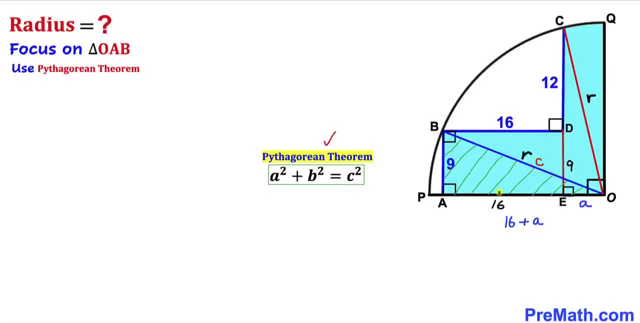 Let me call our longest leg as our side C. This side is C, This side is A and this side is lower case B. So let's go ahead and fill in the blanks in this Pythagorean formula. A, in our case, is 16 plus A whole square, plus B is 9 square equal to radius R square. 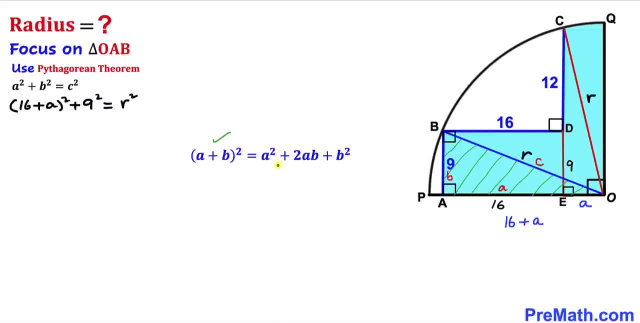 And now let's recall this famous identity: A plus B whole square could be written as A square plus 2AB plus B square. I am going to apply on this binomial, This binomial on the left hand side. So therefore this is going to become 256 plus 32 times A plus A square, and then plus 9 square is going to give us 81, equal to R square. 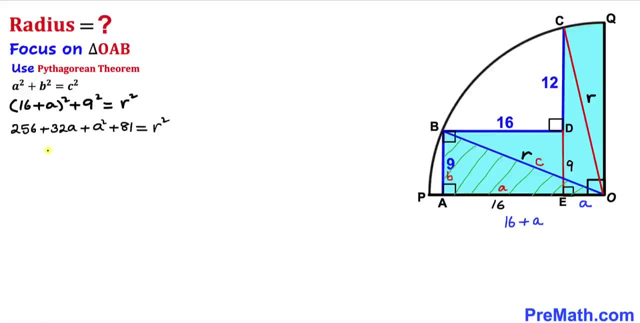 Let's go ahead and combine these like terms. So therefore, this is going to become 337 plus 32.. 32A plus A square equal to R square, Let me go ahead and call this our equation number 1.. And here's our next step. 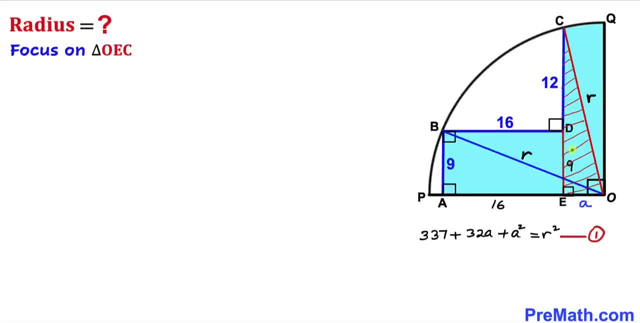 Let's focus on this. another right triangle: OEC. And now let's make an observation. We can see that this whole length, CE, is going to be the sum of 9 plus 12. That is going to become 21.. So, therefore, our CE length turns out to be 21.. 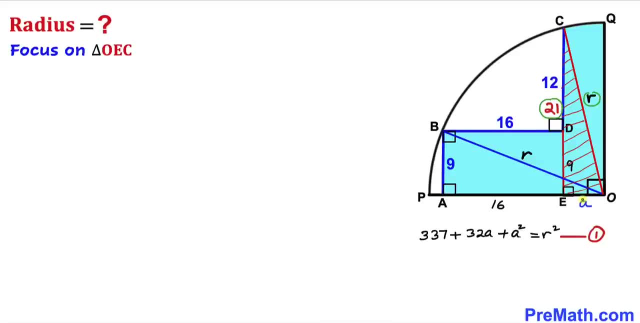 This radius OC is R And this side length OE is A. Now let's go ahead and apply the Pythagorean theorem on this triangle as well. And here's our Pythagorean theorem once again. So, therefore, our longest leg is going to be this radius R. 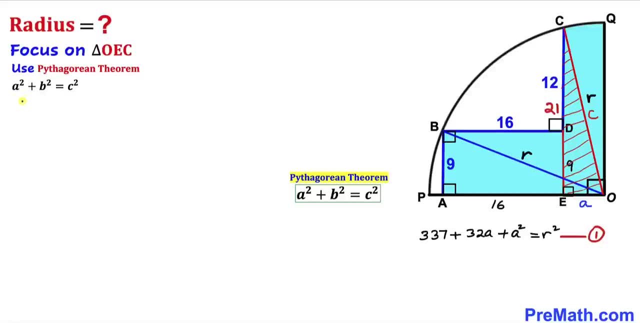 So let's go ahead and fill in the blanks in this Pythagorean formula. A, in our case, is A square Plus B is 21 whole square equal to R square. So let's go ahead and simplify. This is going to become A square plus 441 equal to R square. 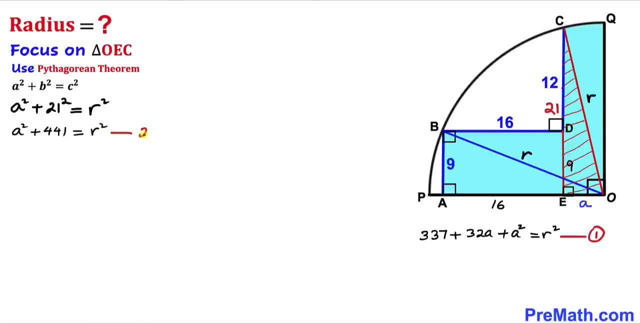 Let me go ahead and call this our equation number 2.. And here we are ended up with these equations 1 and 2.. And now we are going to compare these two equations. We can see, in these two equations, the right hand sides are exactly same. 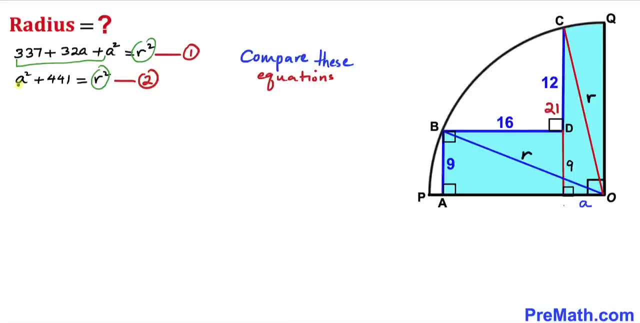 They are identical. So therefore we can equate the left hand sides as well. So therefore we can write 337 plus 32 times A, plus A square equals to: on the right hand side, We are having A square plus 441.. And here we can see that. 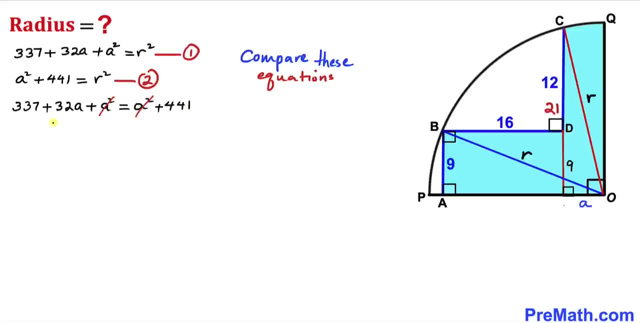 We can see A square and A square. they are gone, So therefore we are ended up with 337 plus 32A equals to 441.. Let's go ahead and subtract 337 from both sides. This is gone, So therefore 32A turns out to be 104.. 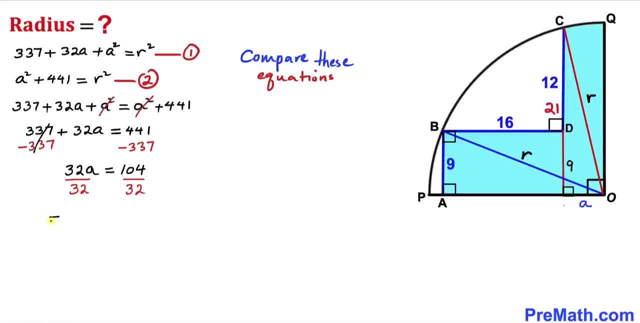 And now let's go ahead and divide both sides by 32.. So, therefore, Our A value turns out to be: if we reduce the right hand side, that is going to give us 13 divided by 4.. And now, since we figured out our A value as 13 divided by 4.. 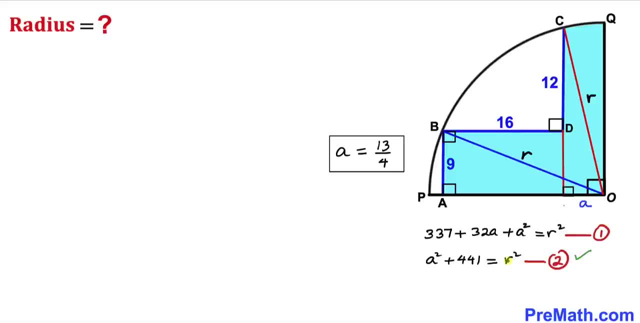 And now let's recall this equation 2 to solve for radius R, And here I have copied down this equation: 2.. A square plus 441 equal to R square, And we know our A value is 13 divided by 4.. So therefore, 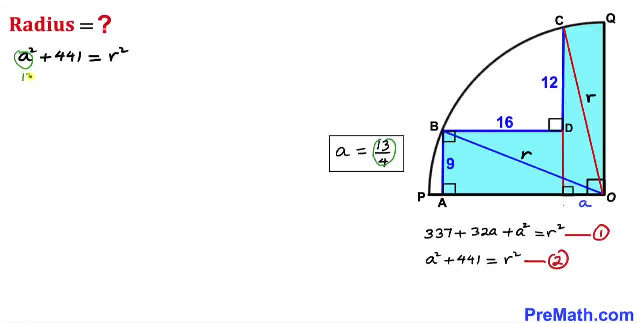 I am going to substitute this: A value, 13 divided by 4, over here. So therefore I can write 13 divided by 4, whole square, plus 441, equal to R square. Let's simplify: that is going to give us 169 divided by 16 plus 441, equal to R square. 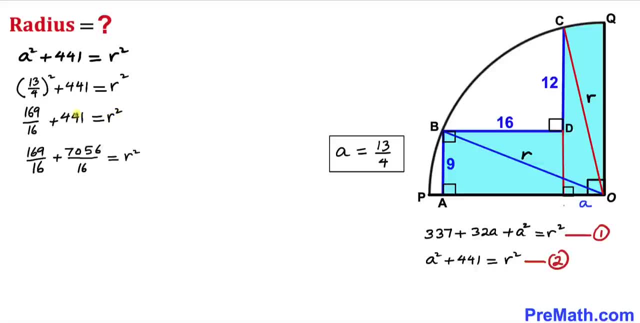 Let's simplify. that is going to give us 169 divided by 4 whole square, plus 441, equal to R square. And here, in this next step, I have multiplied this 441 by 16.. So we got 7056 and divided 16 at the same time. 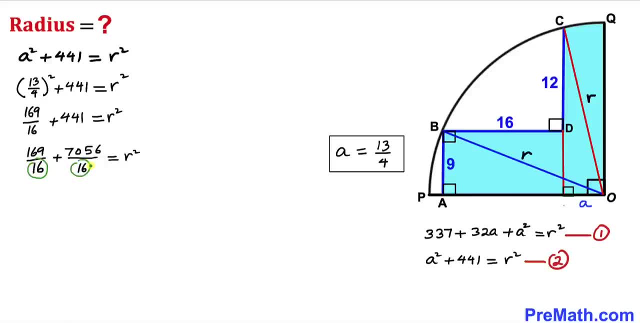 And, as a result, we got the same common denominator. So therefore I can write: 169 plus 7056 divided by 16, equal to R square. So therefore I can write: 169 plus 7056 divided by 16, equal to R square.